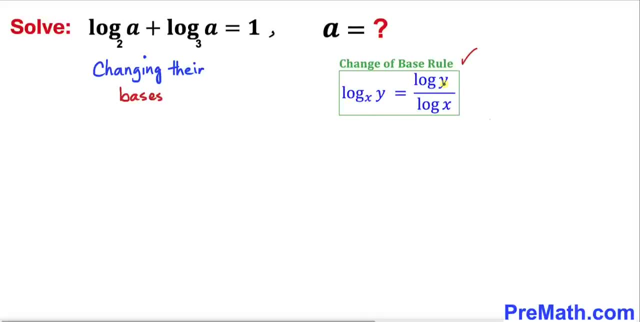 rule: log of y with a base x could be written as log of y divided by log of x. So let's go ahead and apply this change of base rule on this very first term. So this could be written as log of a divided by log of 2 and plus. 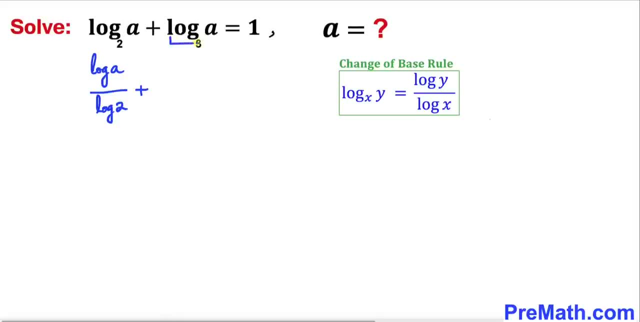 now we are going to apply the rule on this second term, So this could be written as log of a divided by log of 3 equals to 1.. And now we can see that log of a divided by log of 3 equals to 1.. 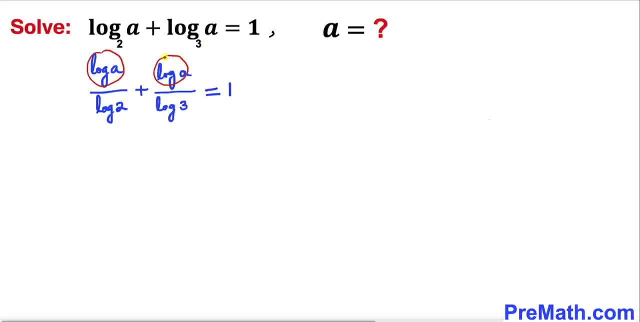 of a and log of a. they are in common so we can factor them out. so therefore i can write 1 divided by log of 2 plus 1 divided by log of 3 times. i am going to put down now log of a that was in common. 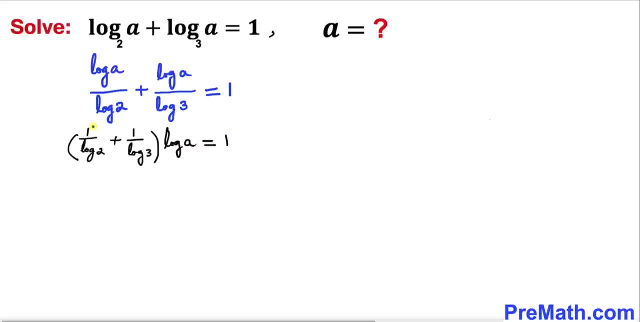 equals to 1, and now let's focus on this part. inside this parentheses- and here i have copied them down- let's go ahead and add these two fractions by crisscross method. so therefore, if we cross, multiply this way, we are going to get 1 times. log of 2 is log of 2. then i'm going to put: 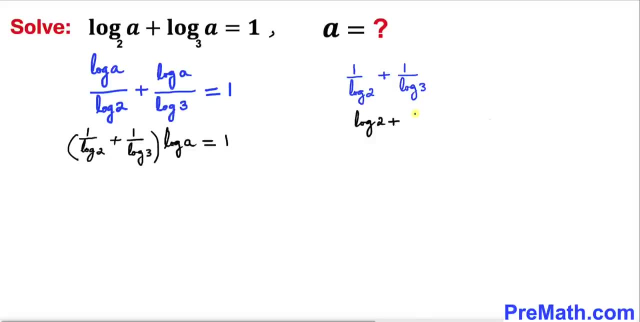 down this plus sign and then 1 times log of 3 is going to be log of 3 divided by. i am going to multiply out these two denominators so i can write log of 2 times log of 3. and now let's recall this product rule we are going to apply on this numerator over here. 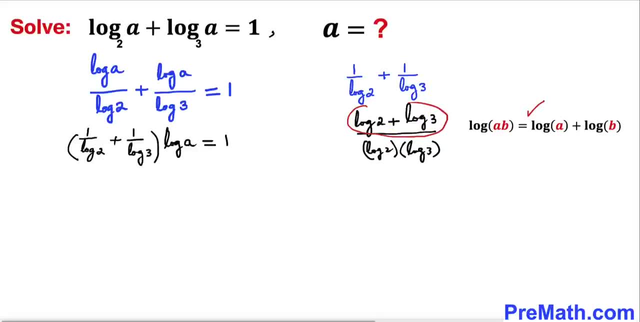 so we can write this one as log of 2 times 3 there, divided by log of 2 times log of 3.. And now we can see that this log of 2 times 3 is going to be log of 6.. So therefore, I am going to replace this whole part by this simplified one. So, therefore, 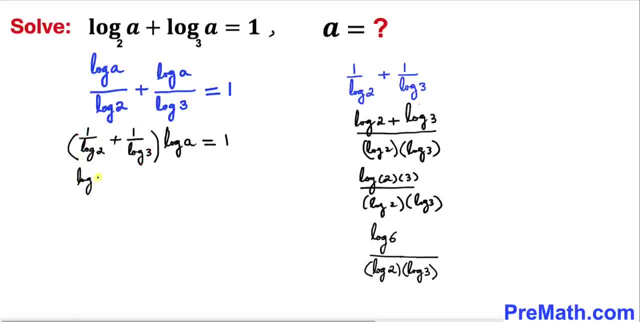 our. this equation is simply is going to become: log of 6 divided by log of 2 times log of 3 times log of a equals to 1.. And now, in this next step, I want to isolate this log of a. So therefore, I am going to multiply by the reciprocal of this fraction. I can write: 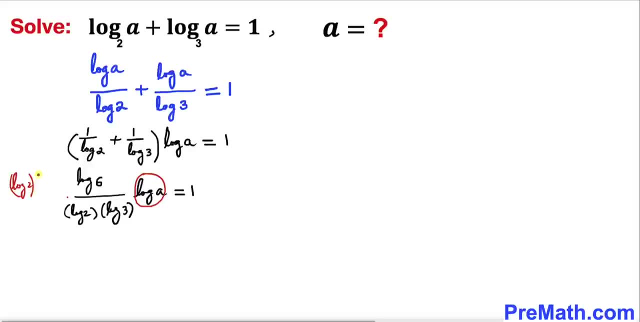 log of 2 times log of 3 divided by log of 6 on the left-hand side, And at the same time I am going to multiply by log of 2 times log of 3 divided by log of 6.. Now we can see that these logs cancel out. This one log of 6 is 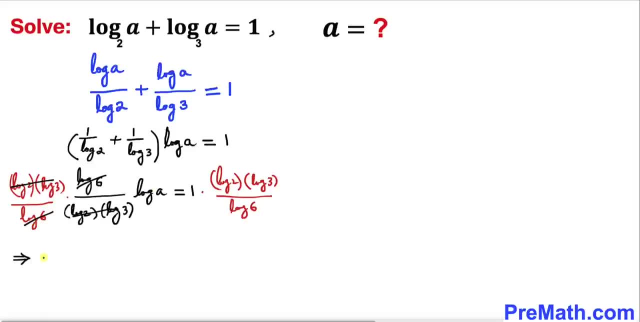 gone with this one, so therefore we ended up with log of a on the left hand side equals to 1 times. this whole thing is going to be log of 2 times log of 3 divided by log of 6.. Now we can see that the basis for all these logs are missing, and just keep in your mind whenever the base is. 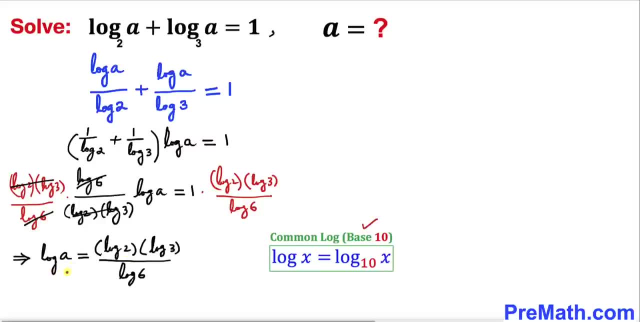 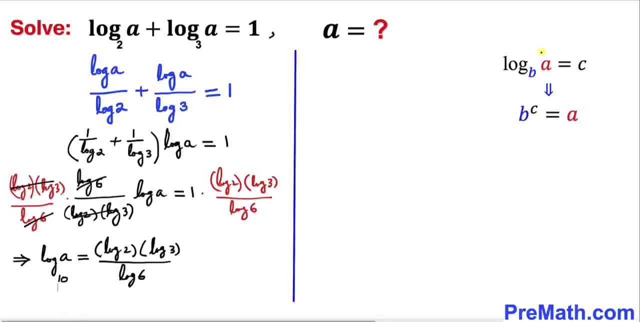 missing. by default. the base is 10 and such kind of logs are called common log, so the base is going to be 10 over here and now. let's recall this conversion rule from logarithmic form to an exponential one. we are going to apply this rule on this equation, so our equation could be: 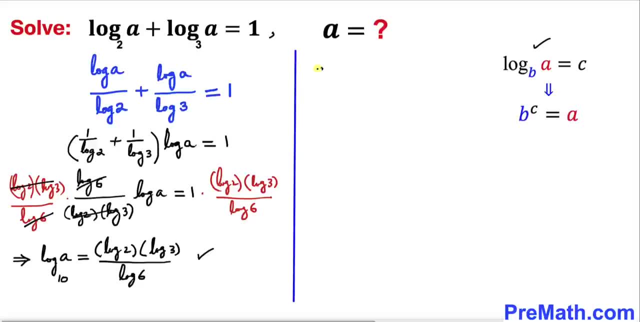 written as this one: in our exponential form, a equals to 10 power log of 2 times log of 3 divided by log of 6. and now we can see that we have isolated our this a. so therefore, this is our solution in terms of our solution. 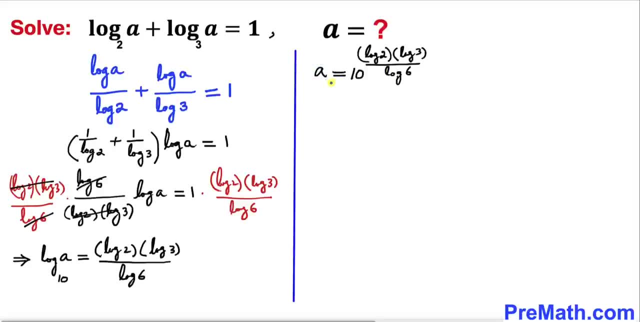 of exponential form. and now I'm going to show you to find the value of a by figuring out this log of 2, log of 3 and log of 6 by using the calculator. Now, if we use a calculator, we can see that log of 2 is approximately equal to 0.301, log of 3 is 0.477 and log of 6 is approximately. 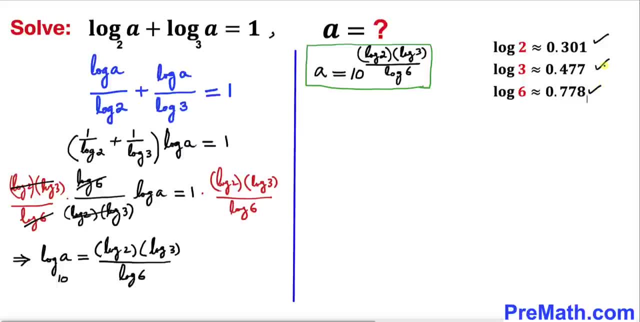 equal to 0.778.. So let's go ahead and fill in the blanks over here. so a equals to 10 power log of 2 is 0.301 times 0.477 divided by 0.778. and now if we multiply and divide this exponent, that will be equal to. 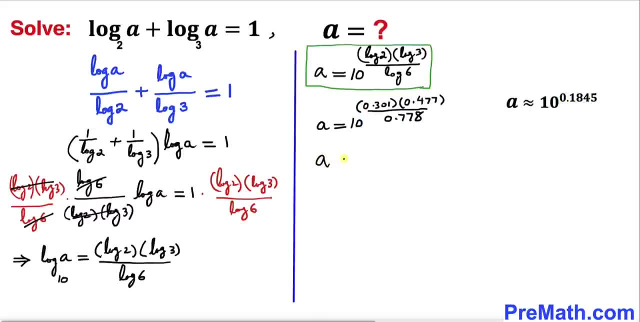 0.1845. so therefore our approximate value of a is going to be 10 power 0.1845. now, if we use a calculator, once again, 10 power 0.1845 is approximately equal to 1.53. so therefore our 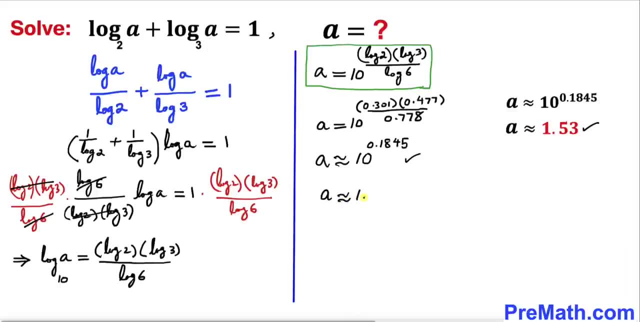 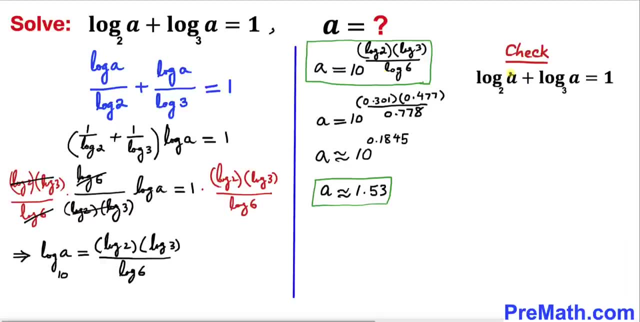 approximate value of a turns out to be 1.53.. And here's our final step. we can check our answer by just plugging in this a value which is approximately equal to 1.53, over here and over here, so the left hand side could be written as: 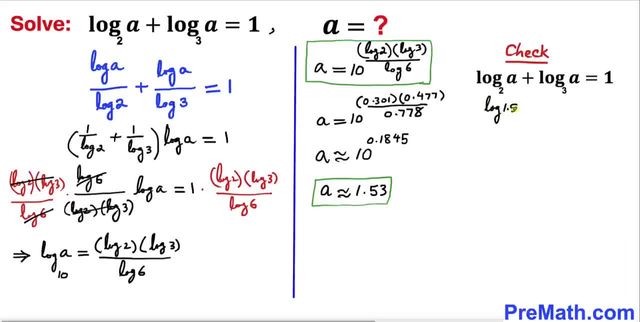 log of 1.53 with the base 2 plus log of 1.53 with the base 3. the question mark is: is it equal to 1? and now, if we plug it in these values in any scientific calculator, we can see the left hand side is indeed equal to 1 and the right hand side is indeed equal to 1. therefore, 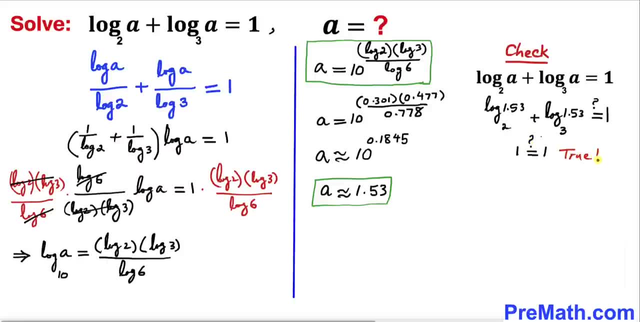 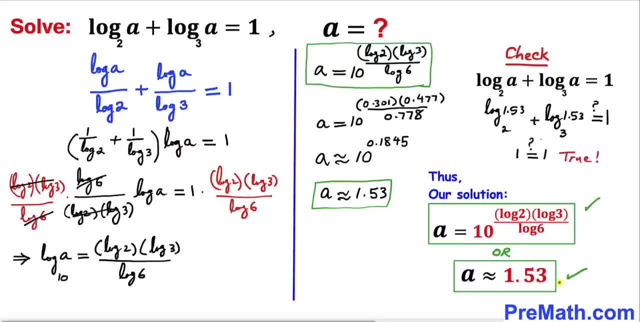 we can see that this is indeed a true statement. so therefore, we conclude that this 1.53 is our valid solution, and thus here's our solution in terms of exponential files. Thanks for watching, and please don't forget to subscribe to my channel for more exciting videos. Bye.